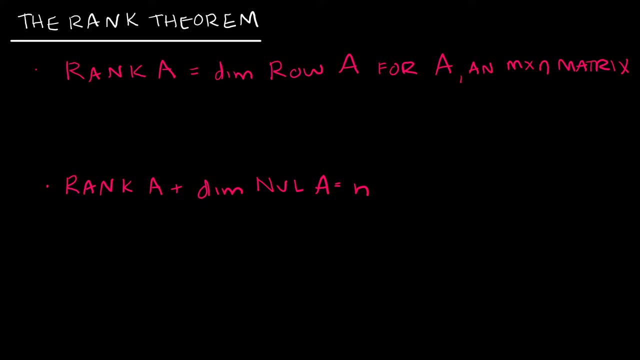 is telling us. The first part of the theorem says that rank of A- which, remember, just means the dimension of the column space of A, is equal to the dimension of the row space of A. So for this is for just an m by n matrix, which is what we're always really talking about. 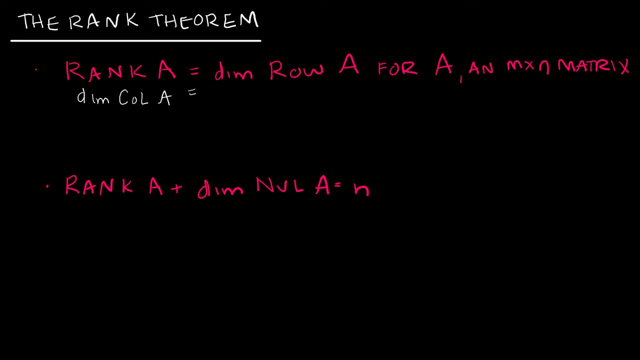 So how is that true? Well, let's recall that the dimension of the column space of A is equal to the dimension of the row space of A. The column space of A is equal to the number of pivot columns. We just refreshed our memories of that a few moments ago, and we know that. 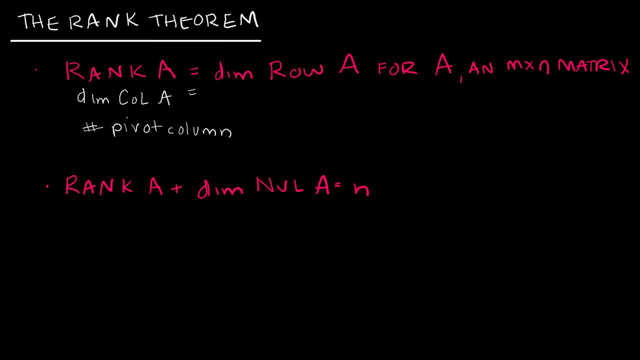 that since that's the number of pivot columns, then for every pivot column there must be a row that is non-zero. So that means every time I have a pivot column, I also have plus one non-zero row. Every pivot needs to have a row. Therefore it makes sense that every time I 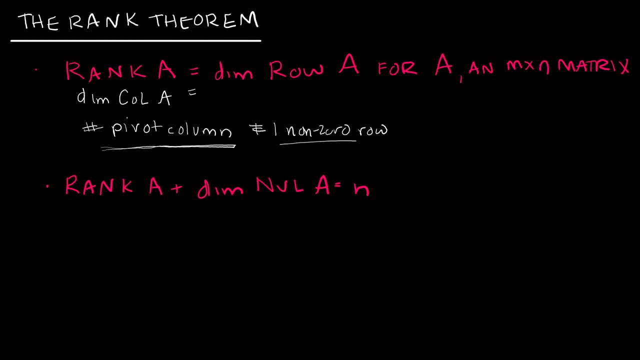 have a pivot column. I will also have a non-zero row which adds to, obviously, the dimensions of the row space of A. Now, if you thought that was easy, this one is even easier. So, this one is even easier. So this one is saying that the rank of A, which again means the dimension of the column, 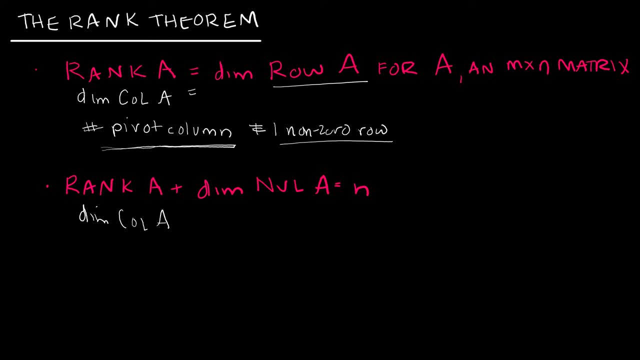 space of A plus the dimension of the null space of A is equal to n. So, if you'll recall, when we learned about dimension, we said: well, the dimensions of the column space of A is just the number of pivot columns and the dimension of the null space of A is the number of free variables. and we know, of course, that. 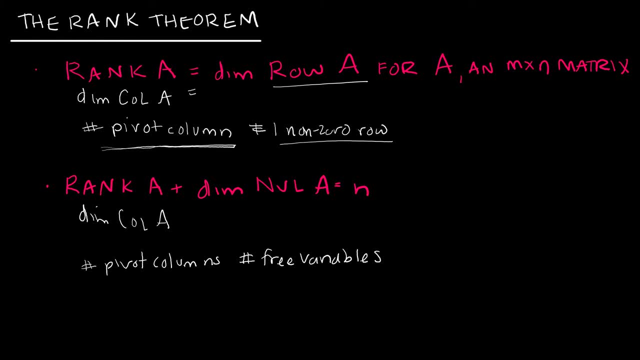 every column is either going to be a pivot column or be a free variable. So it makes perfect sense in an m by n matrix, where n is the number of columns that those are going to add to the total n number of columns. So again, no, that's not a proof, but it's very intuitive. That's supposed. 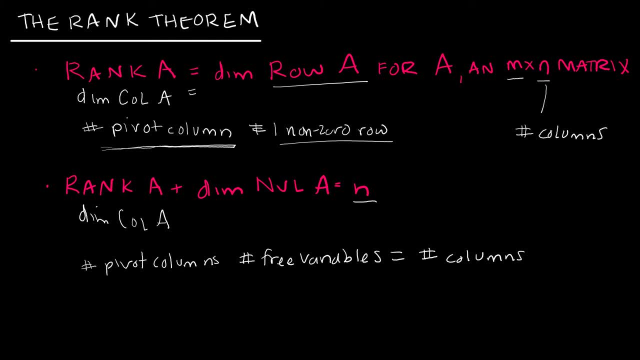 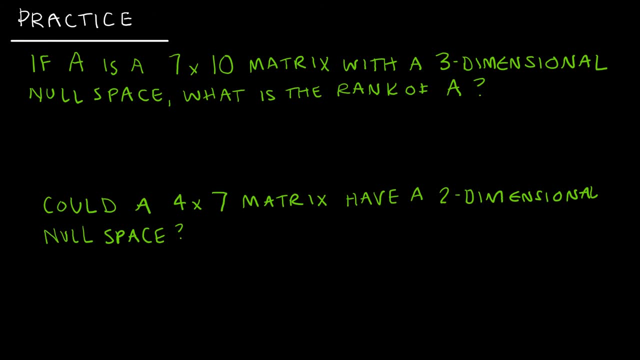 to be a plus. It looks like a t. You get the answer. Let's take a look at a couple of practice. The first one says: if A is a 7 by 10 matrix with a three-dimensional null space, what is the rank of A? Well, this one's very straightforward, We know. 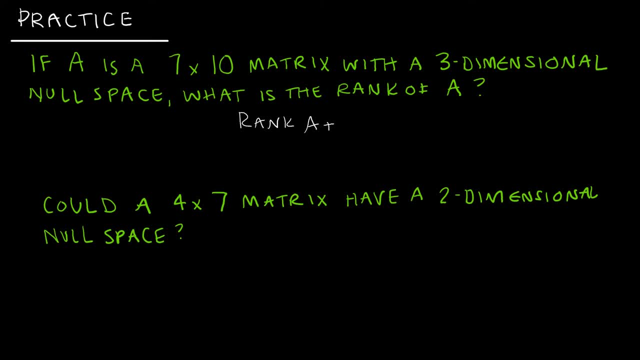 our equation says: the rank of A plus the dimension of the null space of A is equal to n, which is the number of columns in our matrix, which means obviously that the rank of A must be 7.. Good, Next one says: could a 4x7 matrix have a two-dimensional null space? So we're saying: could. 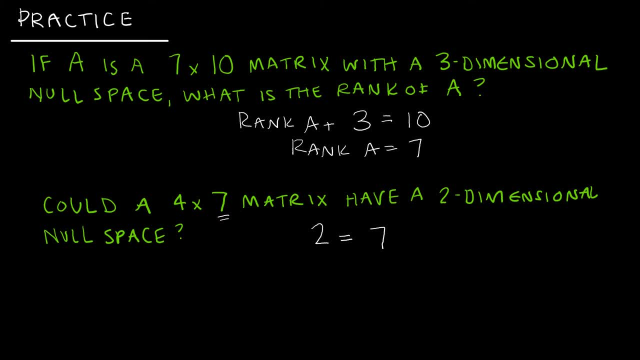 this is going to equal 7. could I have a two-dimensional null space and a rank of 5.. Well, good question. Can I do that? Keep in mind that the columns are vectors in r, 4.. So Could I have 5 here? No, I sure could not, because this is a 4, and therefore this number cannot exceed 4.. 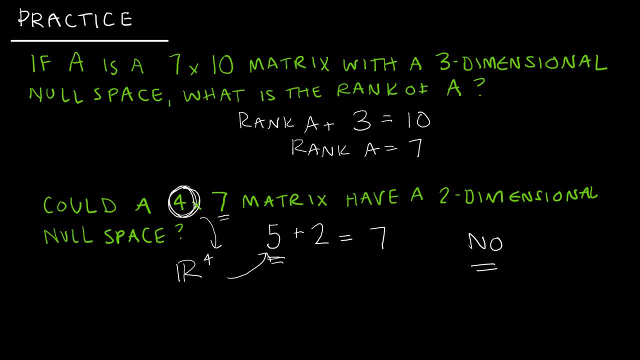 So this would be a no. I cannot have a 4 by 7 matrix with a 2-dimensional null space. I could have a 3-dimensional null space, because now I have 4 plus 3 equals 7. That is okay, but no, I can't exceed R4 in this case. 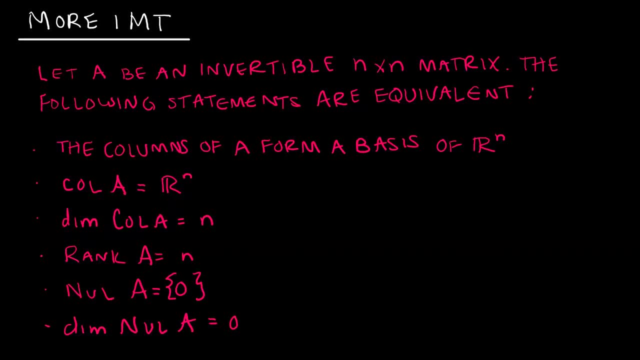 I'm going to leave you with just a little bit more information to add to the invertible matrix theorem. If you'll recall, we learned about that in the last chapter and there were quite a few things that were all equivalent to saying that A is an invertible n-by-n matrix. 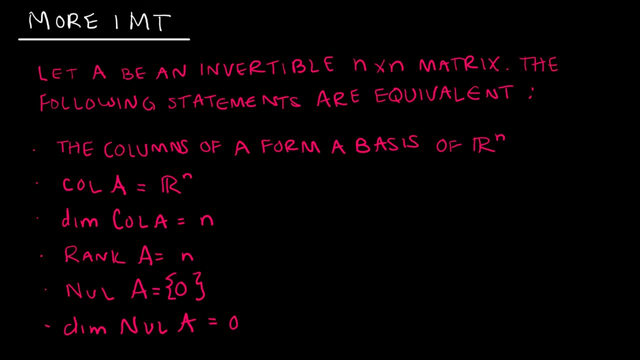 And so now that we know a little bit more about column space and null space and rank and dimension, these are all items that can be added to your invertible matrix theorem And I'm not going to go through them with you or read them through with you. 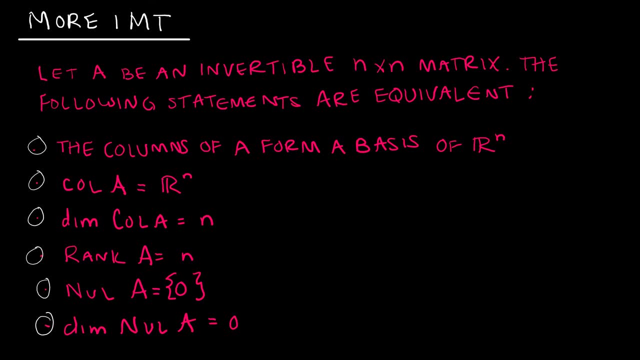 I'm going to let you think about each of those and then, if you have questions about why they are true, you can certainly let me know.